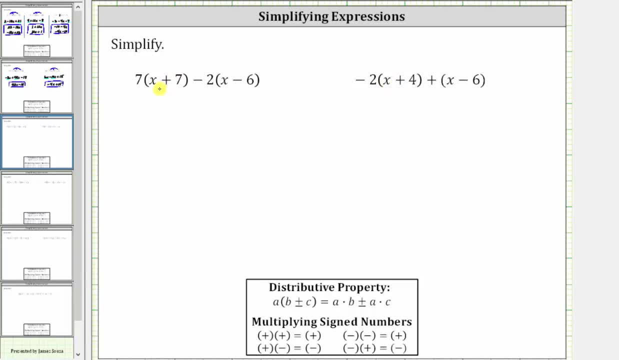 We want to simplify the given expressions. The first expression is seven times the quantity x plus seven minus two times the quantity x minus six. To simplify, we first need to clear the parentheses by distributing and then combine like terms To clear the first set of parentheses. 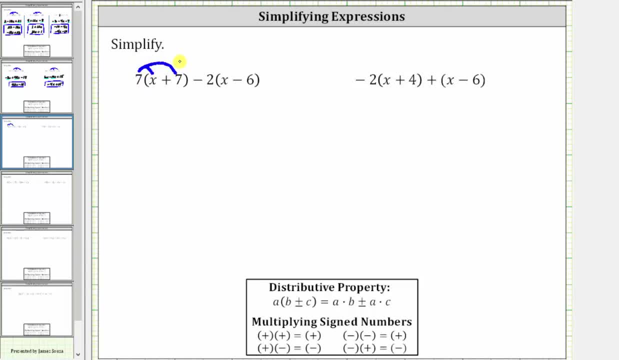 we distribute positive seven, To clear the second set of parentheses, because we have minus two times the quantity x minus six. we distribute negative two. Distributing the seven seven times x is seven x, And then we have seven times seven, which is 49, giving us plus 49. 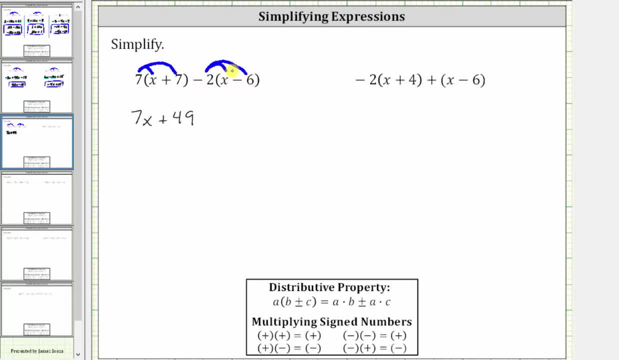 And now we distribute negative two again because of the minus two. Negative two times x is negative two x, giving us minus two x. And then we have negative two times negative six, which is positive 12,, giving us plus 12.. 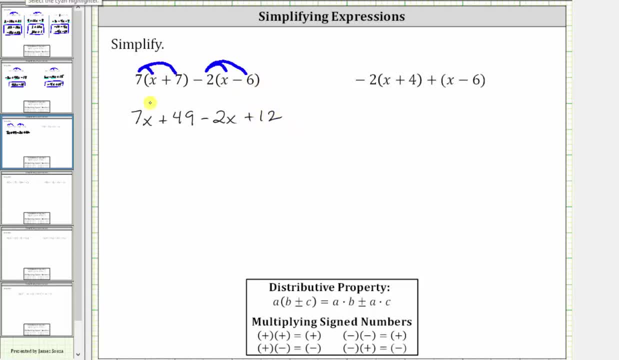 Now that we've cleared the parentheses, we combine like terms. Notice how we have two x terms and we also have two constants: Seven x minus two x is five x, And 49 plus 12 is equal to 61, giving us plus 61.. 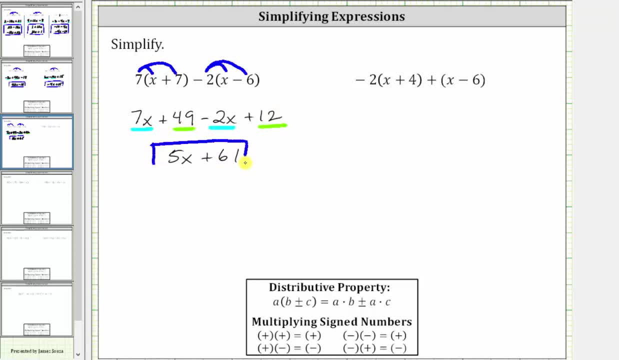 The expression simplifies to five x plus 61.. For the next expression we have negative two times the quantity x plus four plus the quantity x minus six. To clear the first set of parentheses we distribute negative two And notice for the second set of parentheses. 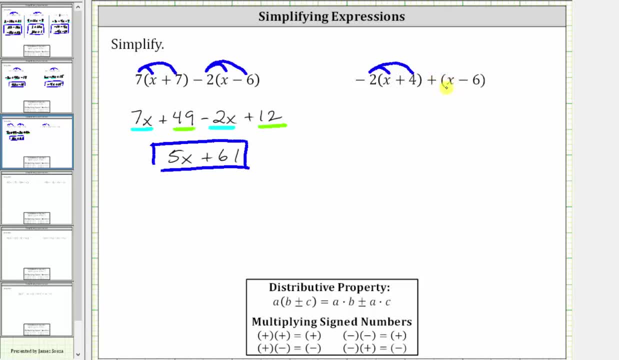 there's no number outside the parentheses And because we have plus the quantity x, minus six, we can just drop the parentheses. Or, if it's helpful, we can think of distributing a positive one, But of course, multiplying by a positive one is not going to change anything. 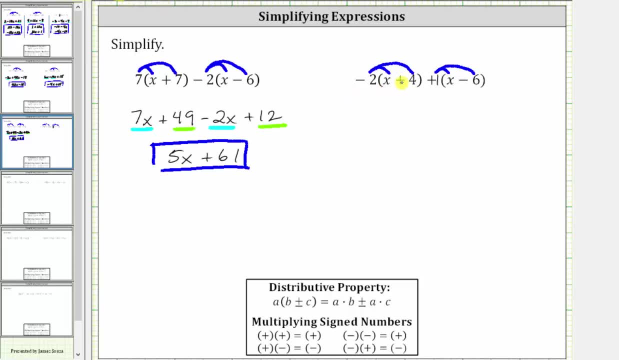 So, distributing negative two, we have negative two times x, which is negative two x x. So we have negative two times x, which is negative two x. So we have negative two times x, which is negative two x. 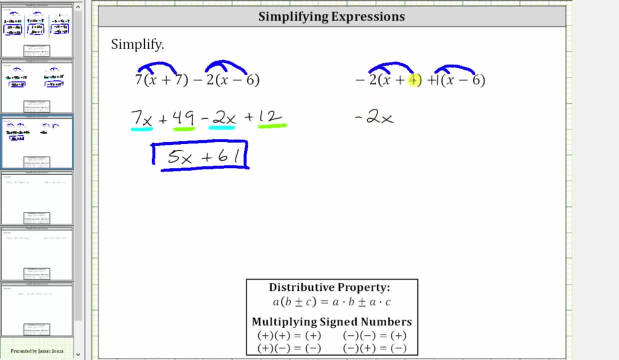 So we have negative two times x, which is negative two x, And then we have negative two times four, which is negative eight, giving us minus eight. And then distributing one just gives us plus x minus six. And now we combine like terms: